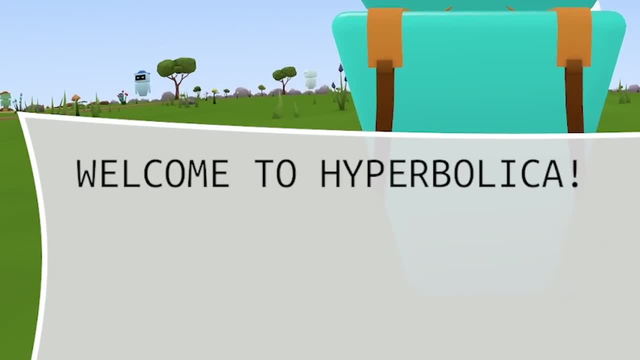 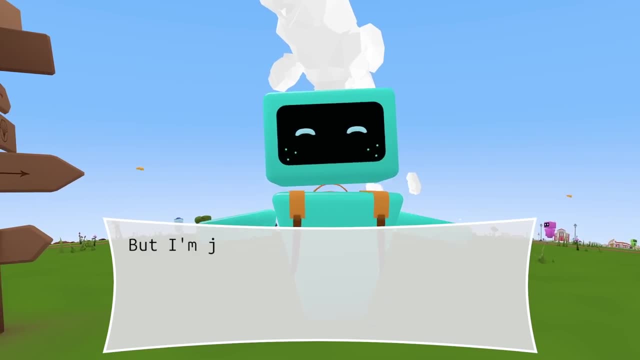 from the virtual learning center. That is correct. Me too. Welcome to Hyperbolica. Oh, that makes sense. It's a hidden world, only for extremely cool people. Yes, okay, So just a warning: if you pick this up yourself, you might not get this level. So yes, it does look like we're on a little planet. 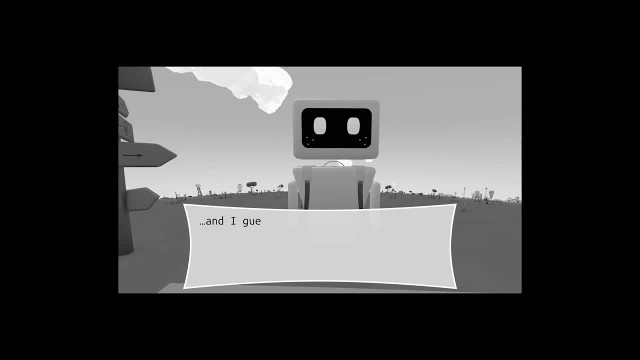 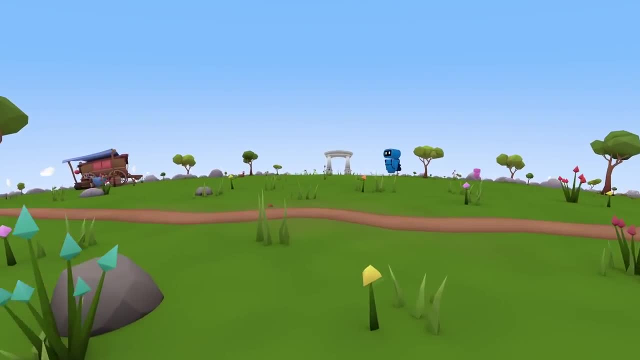 but it's just an illusion. It's really the opposite. Oh, I'm scared. All right, so here we are. Yes, it looks like we are on the world, A little world, But as you walk around, Oh god, it's so weird, It's. 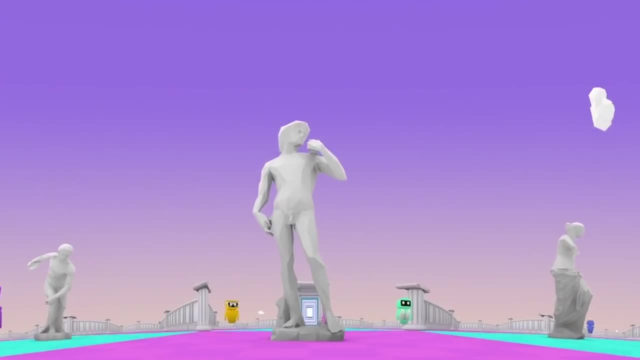 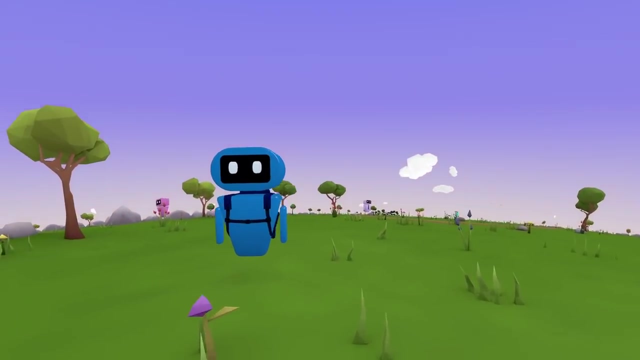 so weird. What's going on? It's like it's far away, but it's not far away. Oh, I don't like this at all. Oh, help me. Anyway, he did actually give us a quest. Oh, I'm tripping balls already. I am tripping balls. 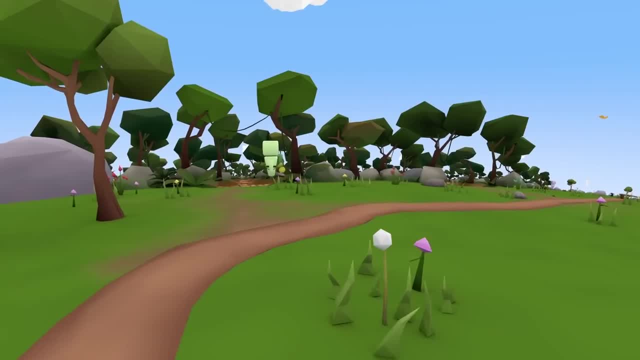 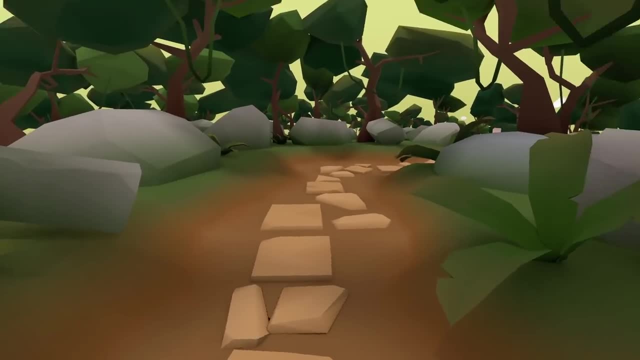 He said: follow this path to the caravan site. So we're gonna follow this path. What is down there? Oh, look at that. I thought it was a little pond thing, but it's actually a huge area. Oh no, this is right, This isn't right. All right, we're just gonna follow this path for now. Where does this path? 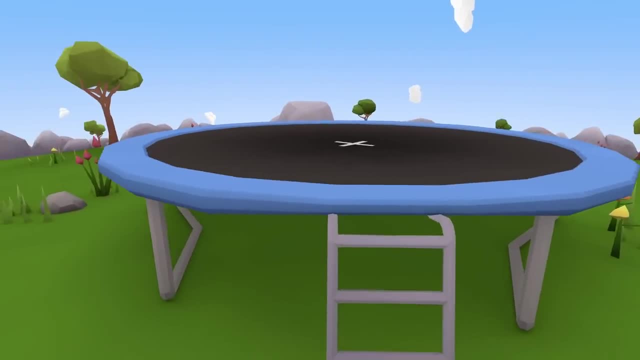 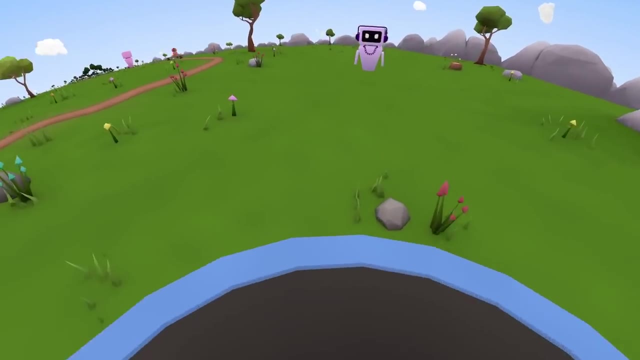 go. Oh, is that a trampoline? That's a trampoline. All right, let's go on the trampoline. Yeah, we're bouncing. Oh look, we're going higher and higher. We can see the entire world. Oh, my goodness, that is. 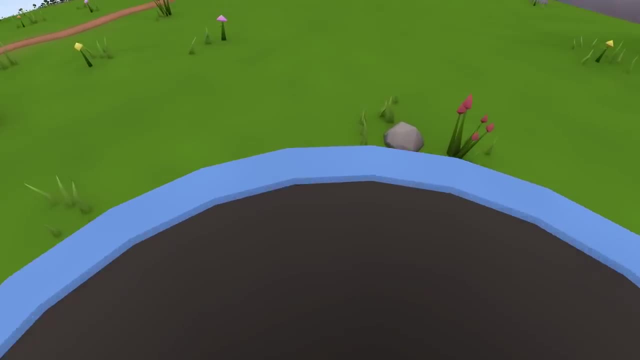 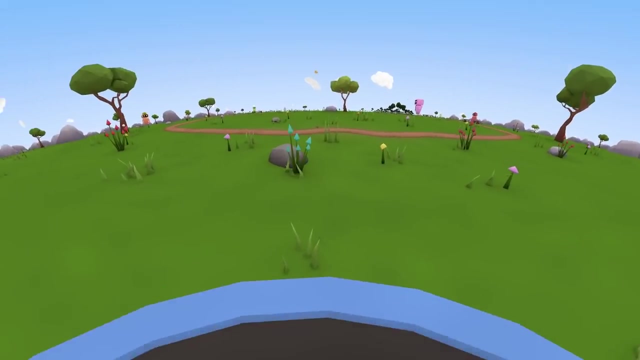 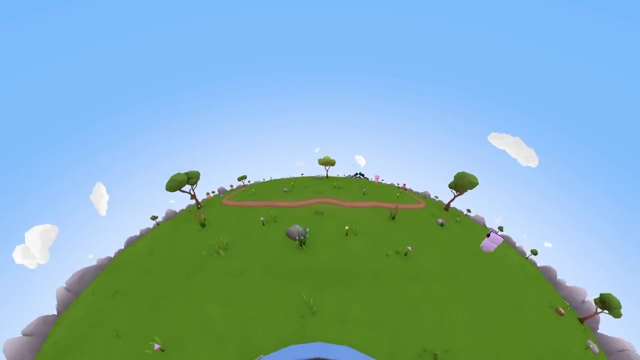 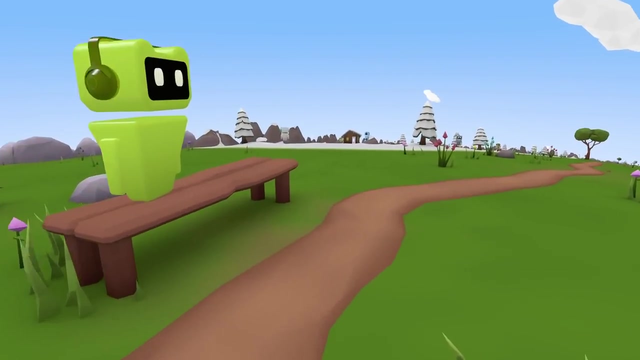 really high, Oh man, the perception is so strange. I am very confused like how someone made this tool. It's like the computer did mushrooms before it rendered the level or something Right, let's bounce off this, Oh god. And, by the way, this game is also VR compatible, so you could be tripping. 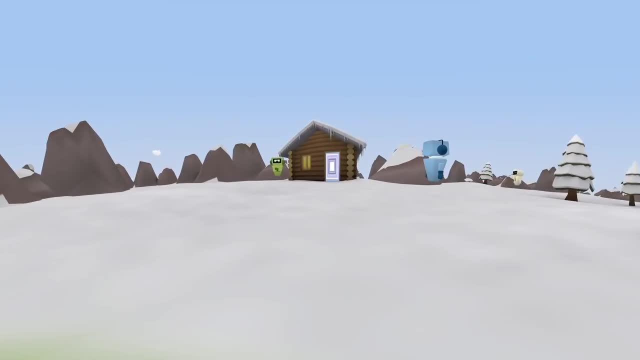 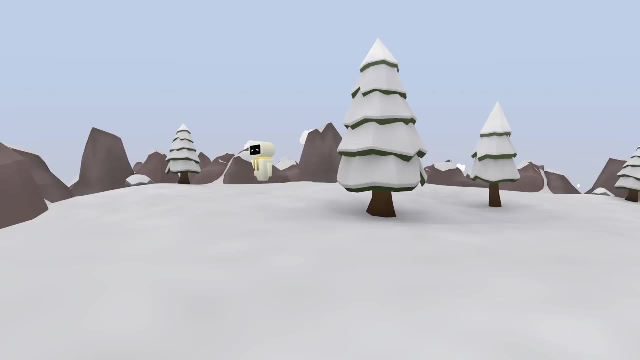 balls and probably vomiting. There's a house over there, So shall we go have a look. It's got a very, very trippy door. What does this guy say? Oh, there's a war in there, We can't go in there yet. 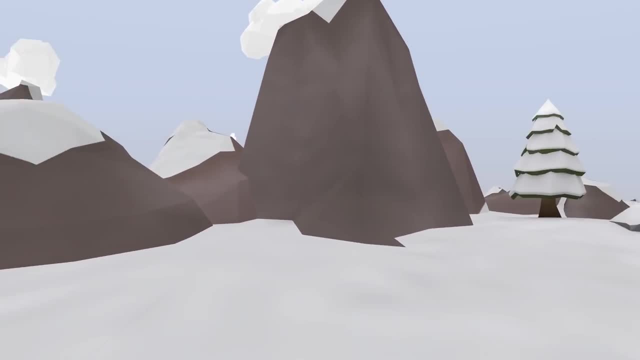 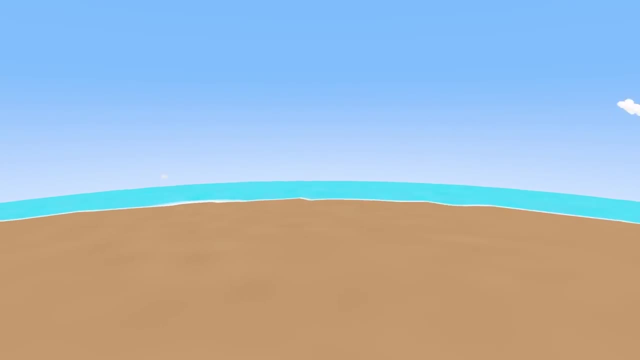 Oh man, it's so weird. It's like these are like painted on, but when you get close, they're not painted at all. All right, so we're still following this path, which we've been following for a days. Oh, the beach. So it looks like a painting, but as you get close, it is actually 3D. Oh, and it. 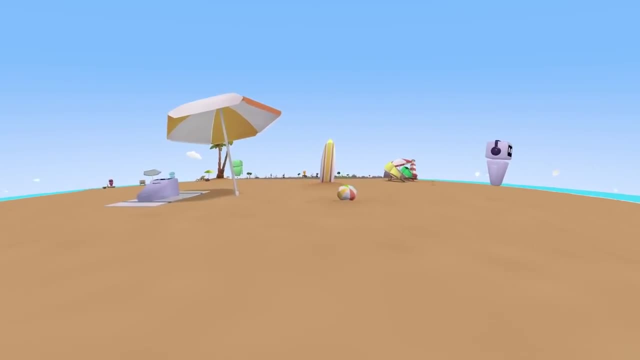 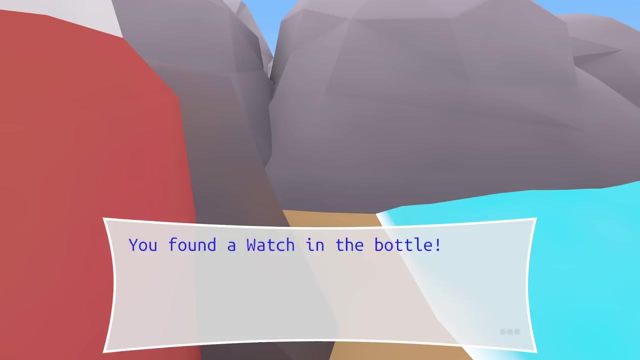 wraps all the way around us. Oh, it's so weird. Why is it so weird? Oh, look at this lighthouse. It is actually a lighthouse. when you get close, Oh, what is this? We found a watch. You found a watch in the bottle, Okay, so yeah, lighthouse. as we walk away, it's gonna. Oh it's so weird, It's so. 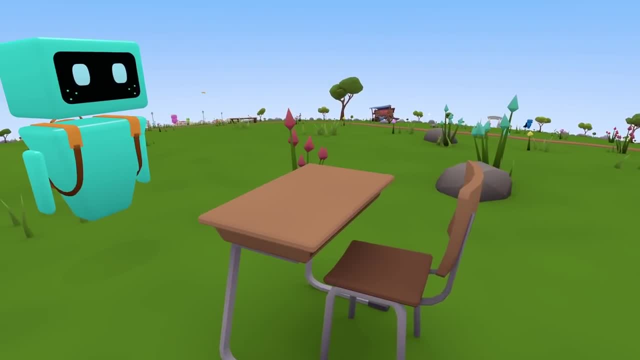 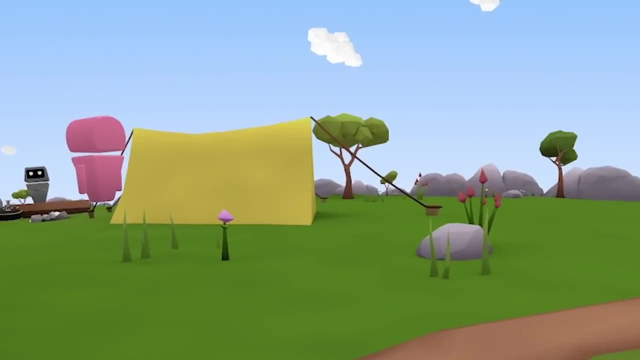 weird. So I'm pretty sure this is where we started. This is the desk, This is the guy we spoke to. There's the sign. So if we go back a bit, here's the path. So we're opposite the beach, So there's. 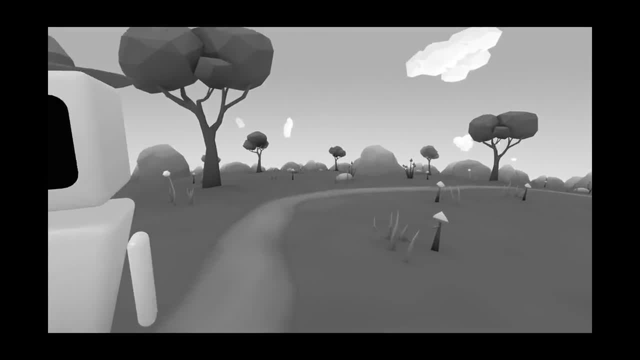 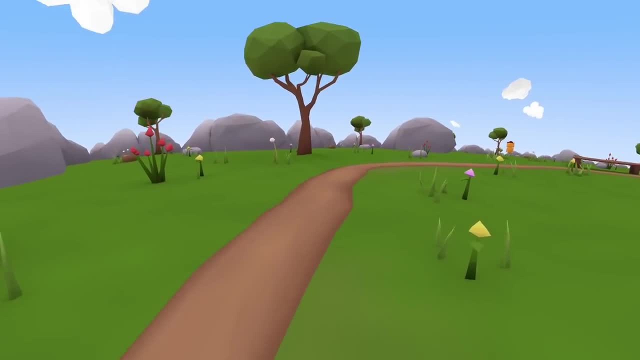 the campers. There's a farm-y thing. I'm tripping balls, So I think we're just going around in circles, are we? What is that? I don't know. Let's keep going around. I feel like the longer we walk, 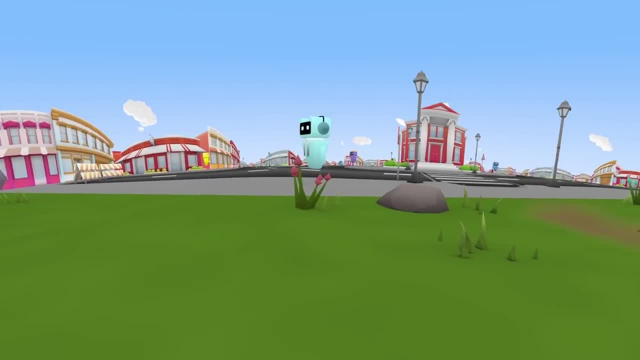 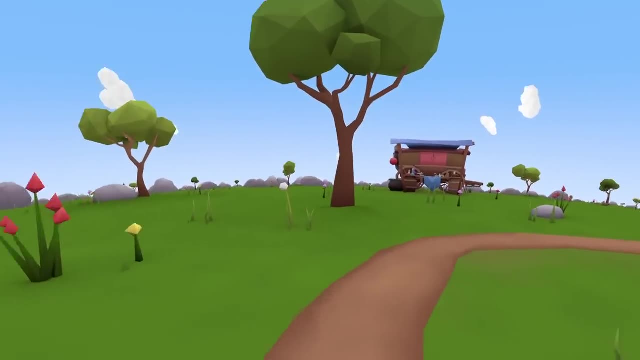 around here. the more different stuff there, Like what? There's an entire city here, but we're still going around in circles. I've done like an entire loop, but there's a city there We're going around Now. there's like a cart thing, Oh, then there's that place. We saw that place like 10 minutes ago. 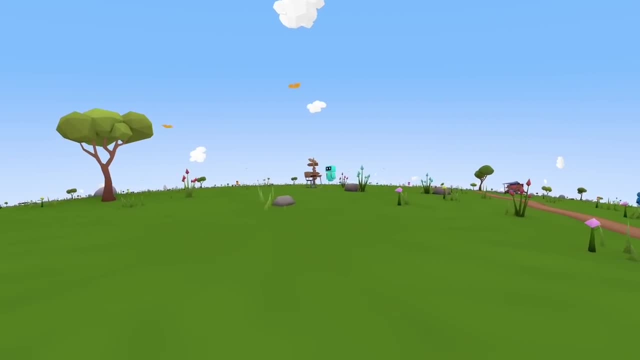 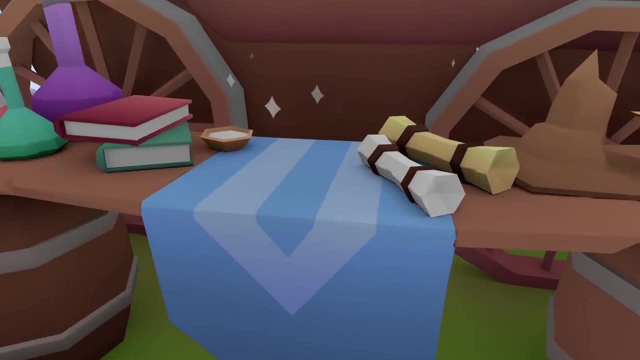 On this path, But this guy's still here. I think it's because the path is longer, depending on- Oh, I don't know. I really don't know what's going on. However, I think this is the caravan we're meant to get to and I think there's going to be a map. Yes, he's given us a map, Right, so we've just been. 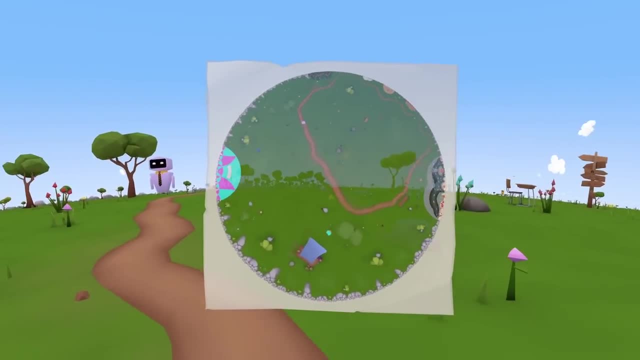 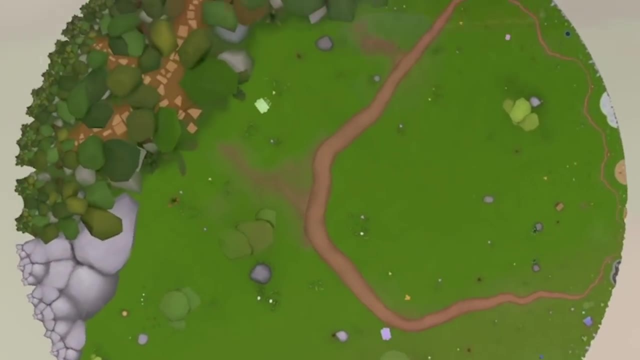 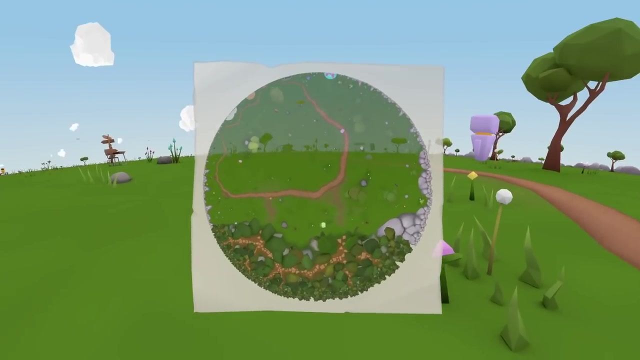 told we're on a quest to find crystals So we can open the map. Oh, and then things get a little bit clearer how it works. So you can see in the center of the map everything's sort of normal. So it's like a fisheye lens, and that fisheye lens actually projects into the real world and therefore it 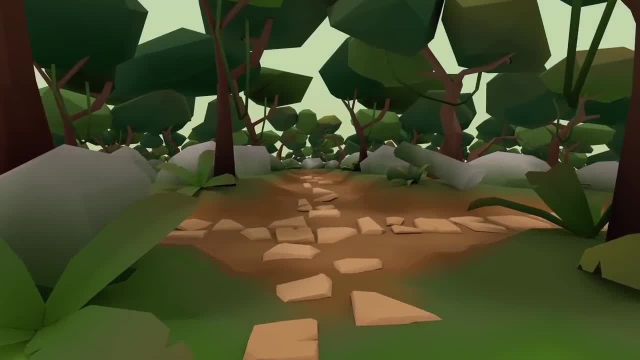 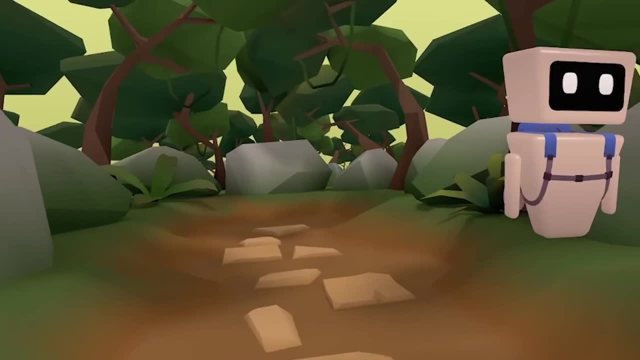 makes you trip balls. So we're going to go in this jungle thing. So we go in here. I'm tripping balls already. We can go. We can't go down any of them. They're dead ends. We can go this way. There's. 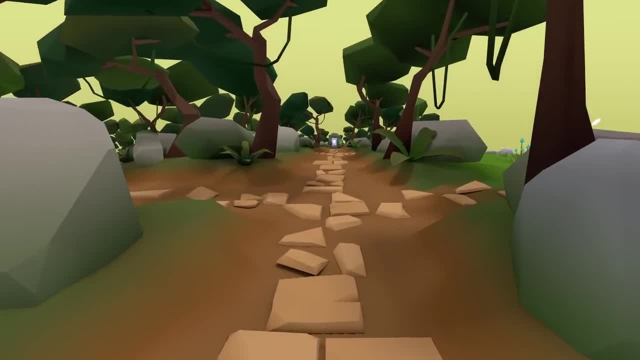 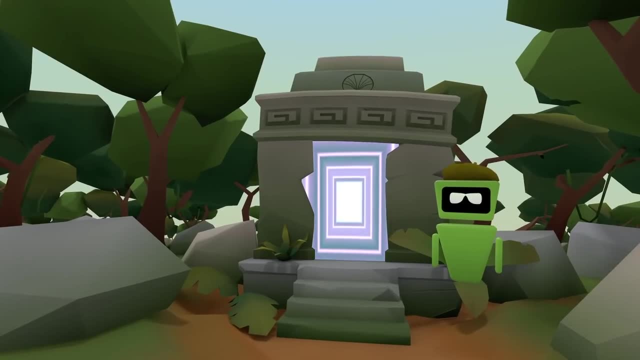 dead end down there. Okay, so two more dead ends and then right should be the way out, But there's actually another turn. Oh god, this thing goes on forever. There is a way out there. That's good to note, All right, and then we got this thing which looks like we're going to trip balls in here. Let's 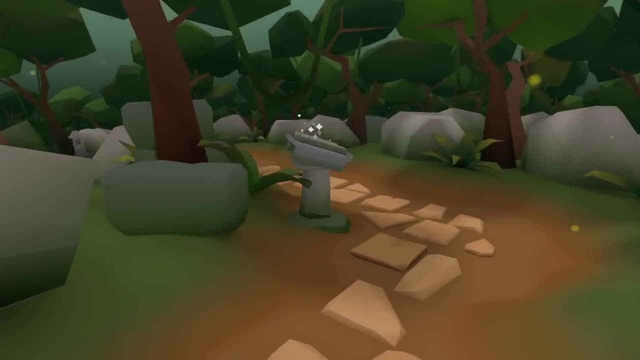 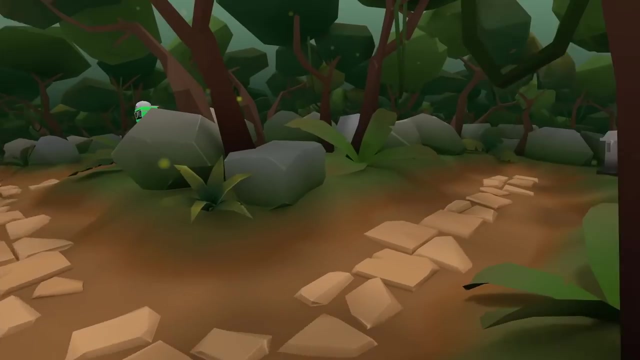 go in Let's see what we got. All right, so where do we go? I guess we go read: what the hell? this is Nothing too important, Just a load of lore. Oh, and now things have already gone wrong because things that were in view you go around a corner and they're no longer in view. All right, this guy's. 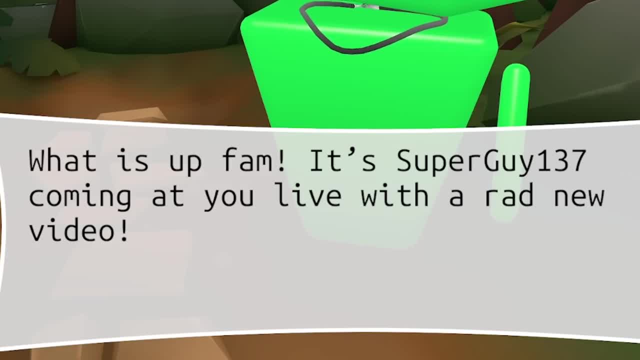 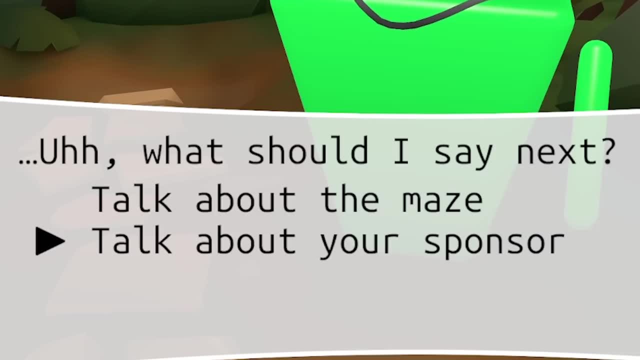 just asked if I could help him out with his YouTube channel. Sure, What is up, fam? It's Superguy137 coming at you with a live and then rad new video. What should he say next? Oh, definitely talk about the sponsor. Gotta make that fat cash. This video is sponsored by Funky Figures Collect. 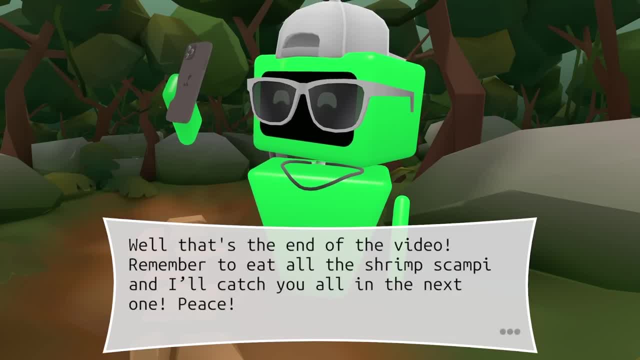 nerdy figurines From all the biggest media franchises. All right, he's just ending his video. Peace. Where's the love and bridges? What an amateur. Anyway, I'm very lost now. How the hell did I get out of this place? 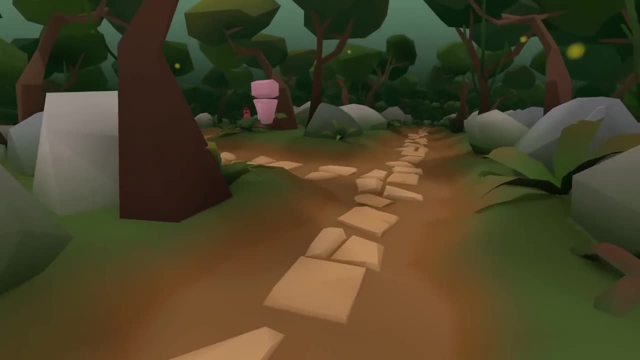 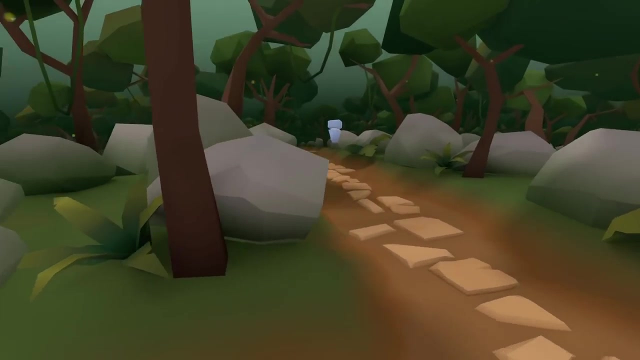 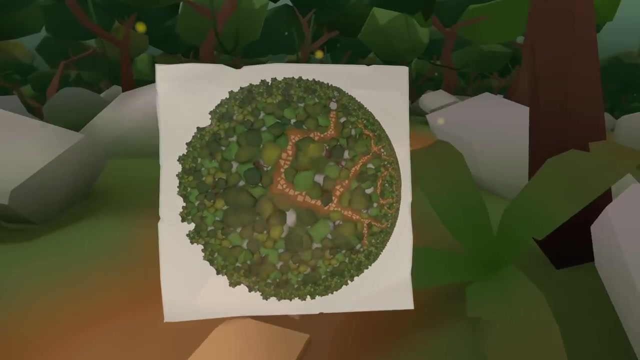 Oh, I'm so confused. There's so many paths. There's so many paths Basically because this exists in like a normal space. I just can't get my head around how this works, Like I'm just going left and left, but then left doesn't exist anymore. I'm so confused. However, thank goodness there is a map. 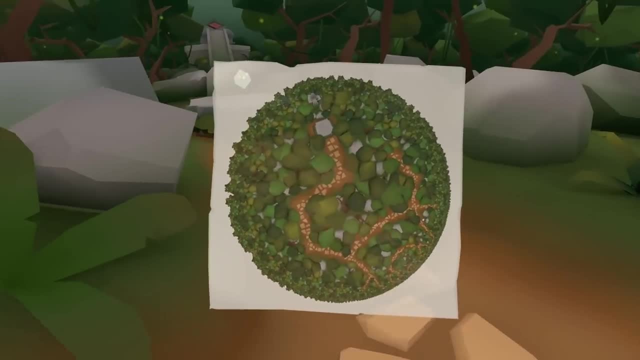 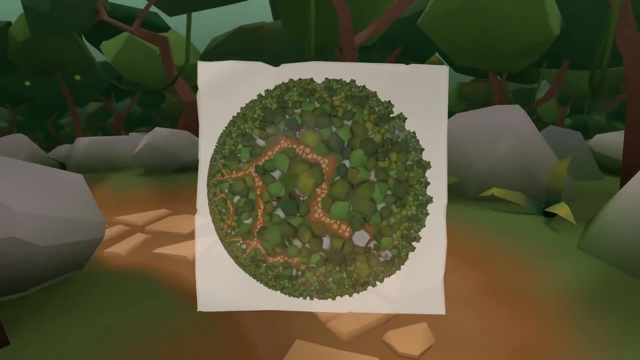 so we can find our way out, A way that our brain can recognize Like: oh, what is this? Is this one of the crystals? I think it's a crystal, but we found the crystal Right. I'm really gonna have to use this map to get back. 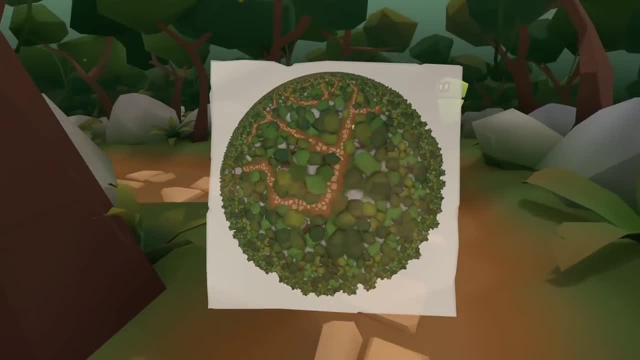 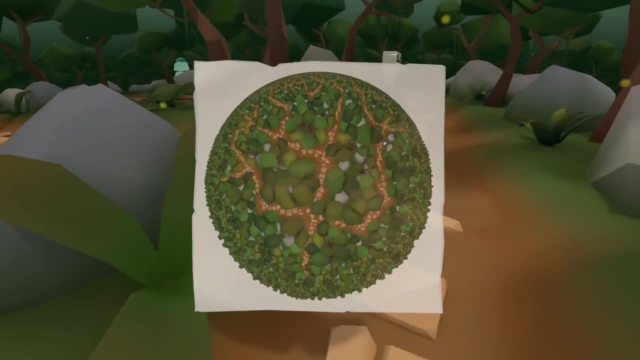 out, Firstly, if I don't want to throw up. Secondly, if I actually want to get out of here. Like it all looks so simple when you're viewing it in this view, Yeah, so basically, I think as you walk along, areas like they change So you can sort of see, like, like that bend straight ahead of me, What is. 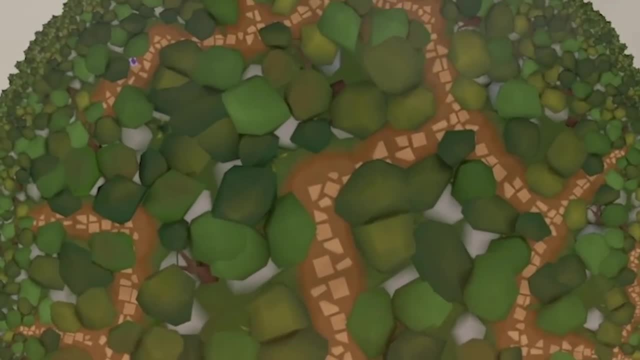 it like 60 degrees, 70 degrees, But as we get close it changes to 90 degrees, So I'm just gonna go with 90 degrees. Oh, it's so confusing. Anyway, we finally found our way out, Alright. so now we've. 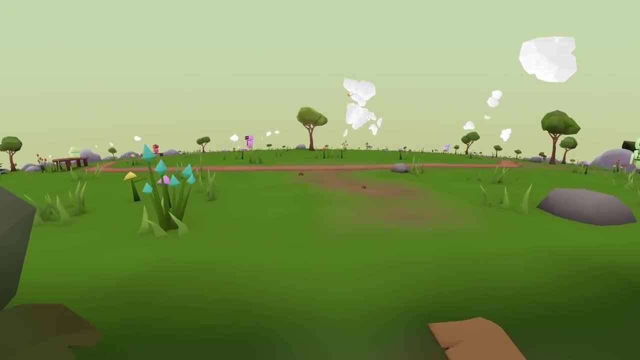 just got to get out of this little bit. I think there's a left here. Yeah, thank god, We're free. We're back on the never-ending path, Alright, so let's see. Can we go in the snowy area now? Yes, 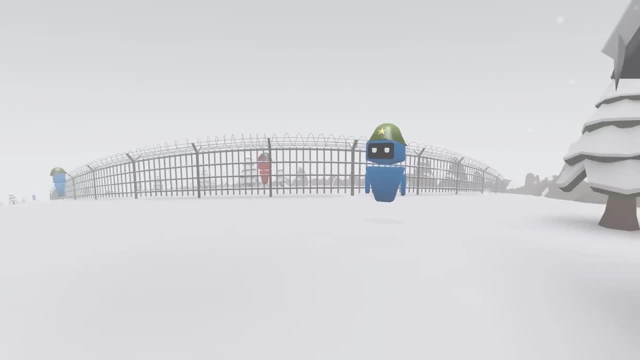 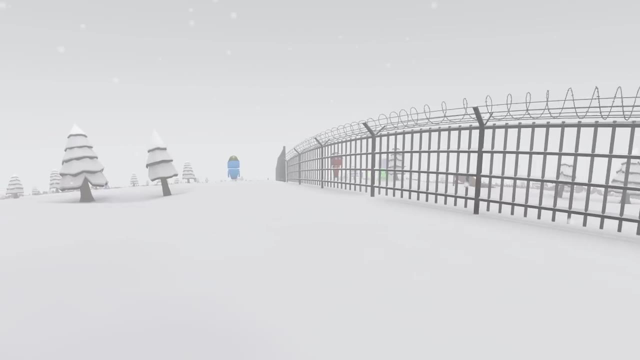 we've just been told there's a ceasefire, We can go in and oh god, look at that fence, Look at that fence. That's not good, Alright. so they just said there's like a war going on, A cold war because it's in the snow, Terrible. This fence is freaking me out a bit, But also actually helping me, because 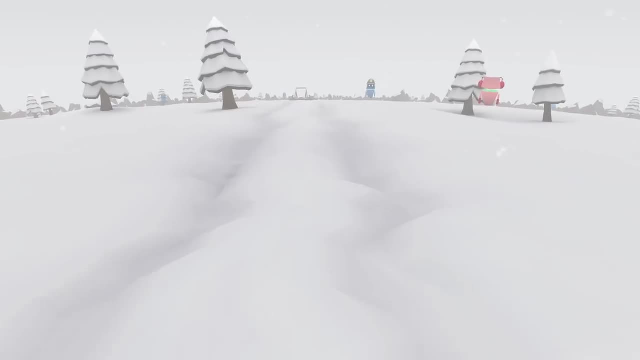 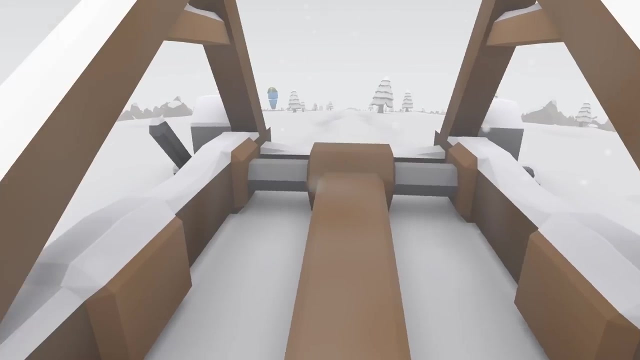 where straight lines go, Assuming it is straight. that is: Oh, let's follow these tracks. What's over here? Is that like? It looks like a catapult or something. I think it is a catapult. Do I get in here? Alright, we're in. Someone fire me. Someone press fire? Alright. okay, here's a cube, I assume. 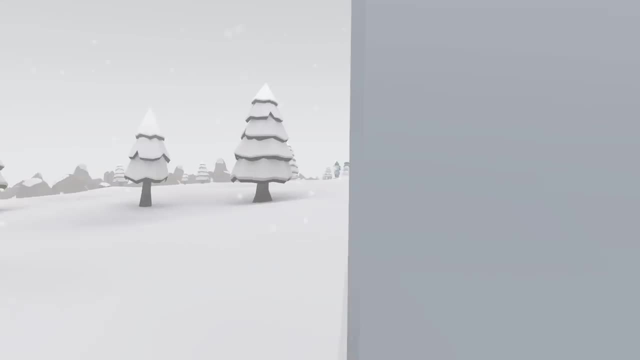 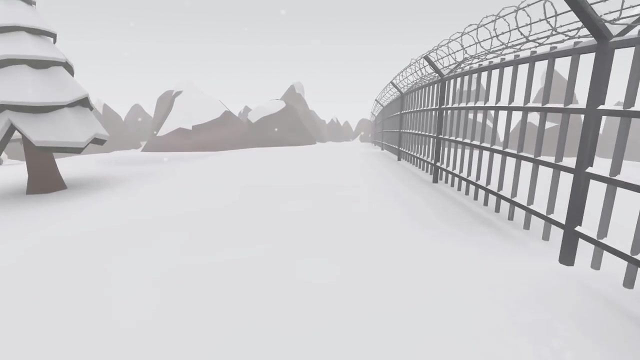 it's a cube. Please be a cube. I'm scared of like going around things in case it's not what I think it is. But okay, that was actually a cube. Thank you, game, for not spinning me out. Alright, let's just keep following this fence. It's got a finish somewhere. Oh, and it does It, actually, does It. 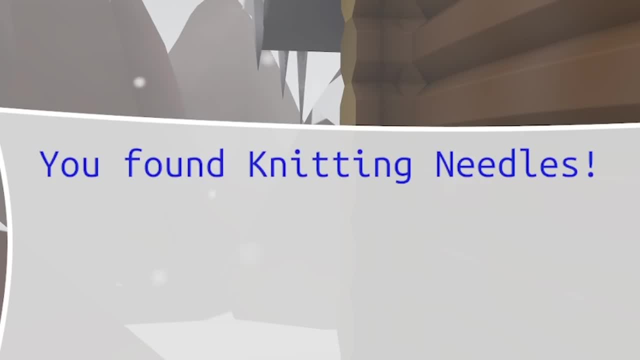 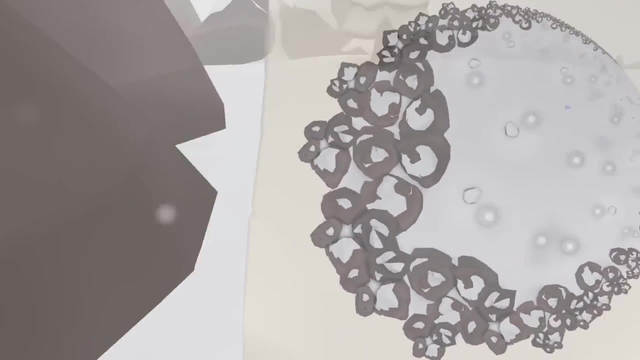 does, Thank god. What the hell are these Knitting needles? Yes, apparently they are Alright. I've been going around the edge of this map for what seems like days. I don't even understand, Like my smooth engineering brain cannot comprehend what's going on really. Oh, it's the YouTube again. Nah. 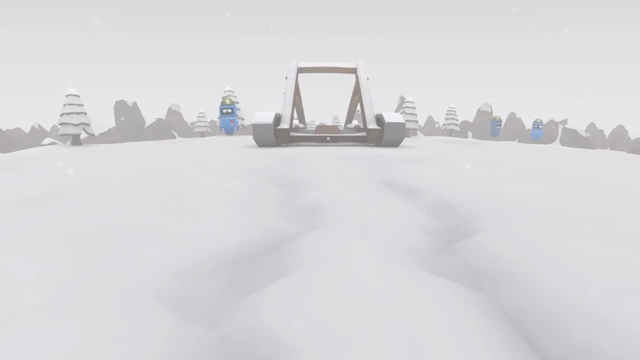 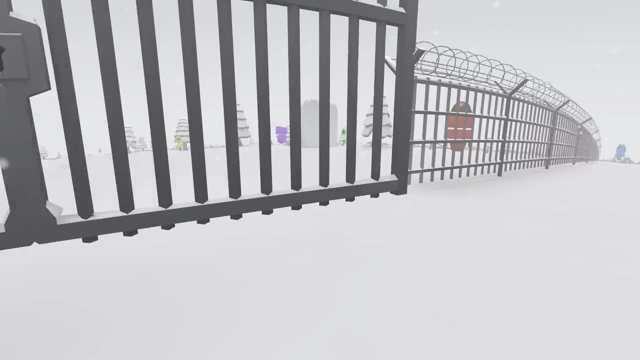 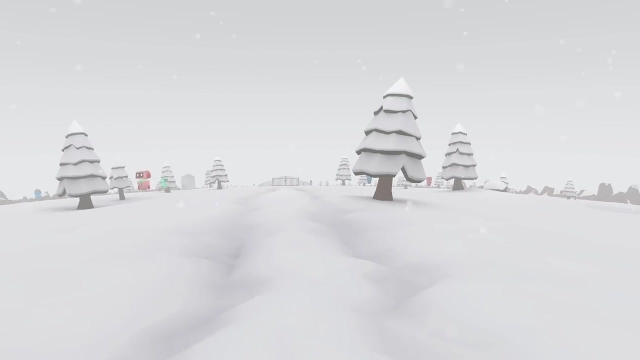 bog off, mate. Alright, we're finally back at the catapult. So, oh, this is really hard to explain, but like, going from that end of the fence to that end of the fence next to the fence takes like 20 minutes, Like by this catapult which isn't too far from the fence. looking at it, It took like 5-10. 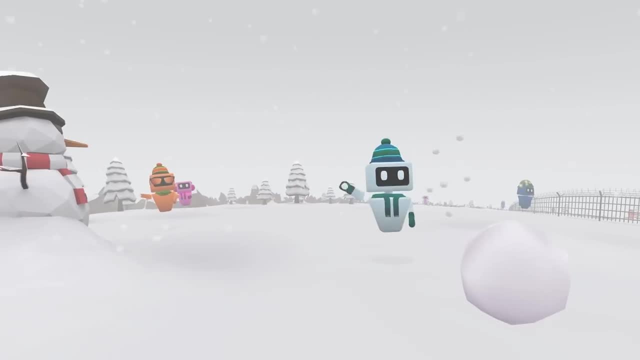 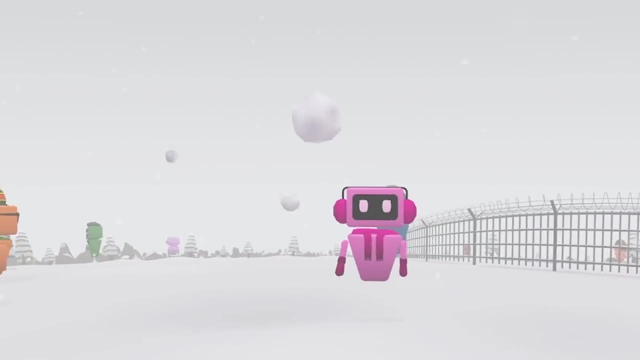 minutes. Alright, we've just been challenged to a snowball fight, So, boosh, eat some of that. Boosh, Oh no, Oh no, things curve, Oh ow, He hit me. Oh, I'm so. This is really, really confusing. I gotta. 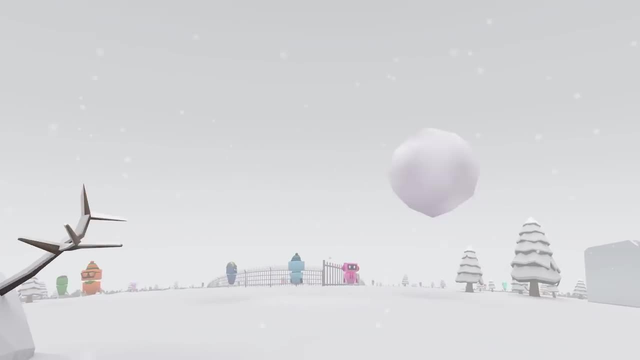 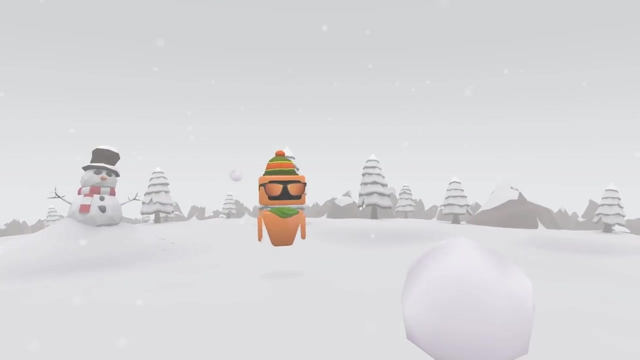 hit each of them five times. Bloody hell, We got that guy. Alright, go for the long rangers. Damn perception. Alright, we got. we got the blue guy- Blue guy's down- Eat some of that pink Alright out. Yes, we did it, Alright. so we've been given a secret password so that we can get catapulted.